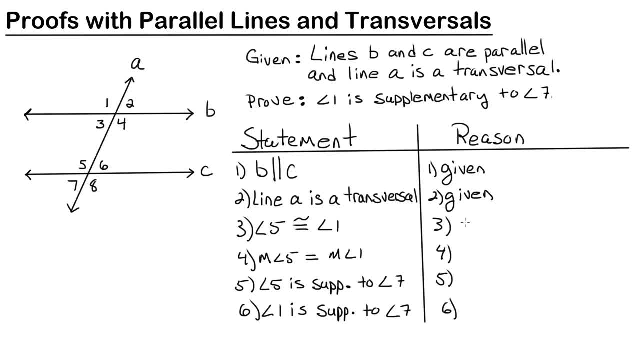 So we know that angle 5 is congruent to angle 1. Because of the corresponding angles theorem. So I'll just do this: for angles theorem, Statement 4, the measure of angle 5 is equal to the measure of angle 1, and since we know that they're congruent, that's how we know they're equal. so that is definition of congruence. 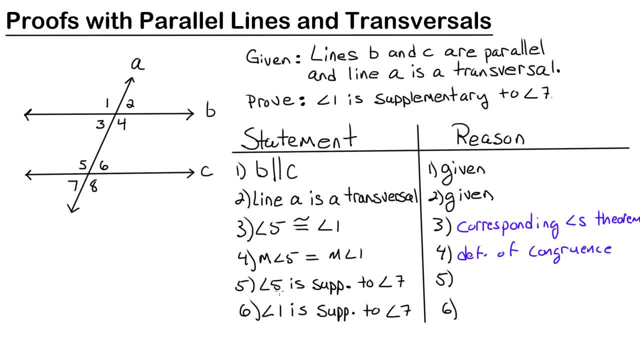 Statement 5 says angle 5 is supplementary to angle 7.. Let's take a look at them: here's 5,, here's 7, and together they make a straight line. So we know their supplementary because they are a linear pair, and that's our reason is definition of linear pair. 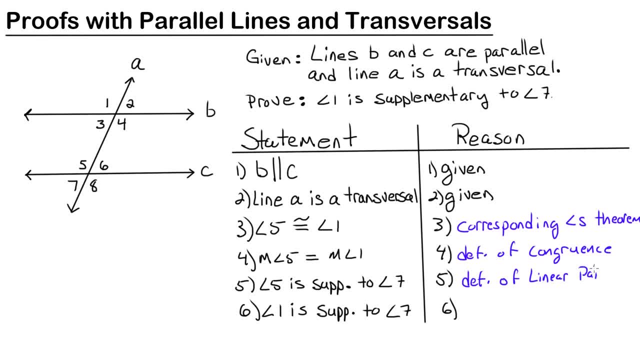 So, finally, if angle 7 and angle 5 are supplementary and if angle 6 are vey similar, then they can't be a linear pair. If angle 7 to angle 5 are supplementary, angle 5 is congruent with angle 1. that means that angle 7 and angle 1 are also supplementary. 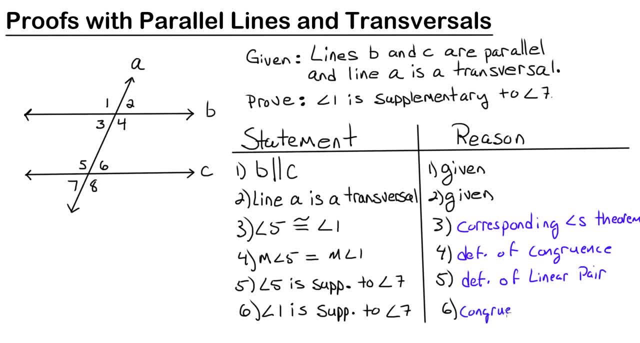 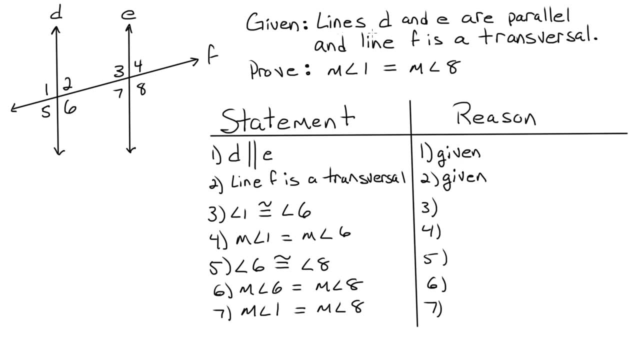 and that is called the congruent supplements theorem. So our next example says: given lines D and E- here they are- are parallel and line F is a transversal prove that the measure of angle 1 is equal to the measure of angle 8.. So let's look at our statements and reasons. number one, D, is: 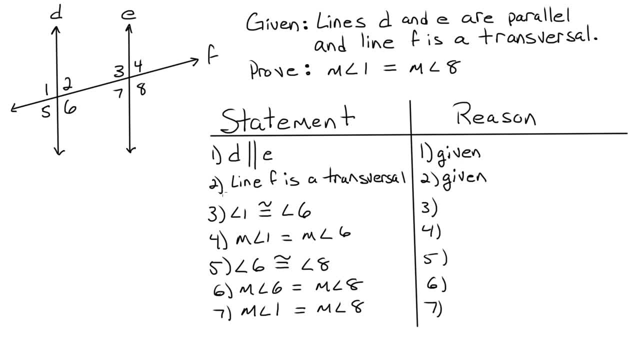 parallel to E. that's given. number two: line F is a transversal. that is also given. Statement 3: angle 1 is congruent to angle 6. if we look at them we can see that they are vertical. so we know they're congruent because of the vertical. 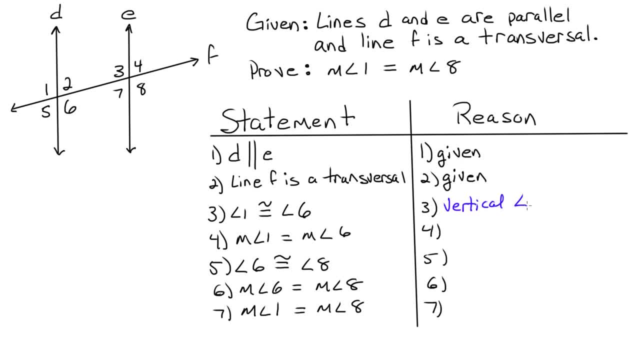 Angles theorem. and since they are congruent, we know that the measure of angle 1 is equal to the measure of angle 6. so that is the definition of congruence. Statement 5 says angle 6 is congruent to angle 8 and we see that that is because they are corresponding, so that 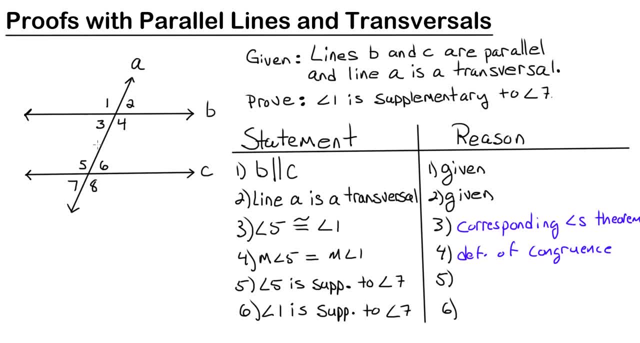 Statement 5 says angle 5 is supplementary to angle 7, let's take a look at them: here's 5, here's 7, and together they make a straight line. so we know they're supplementary because they are a linear pair, and that's our reason is definition of linear pair. 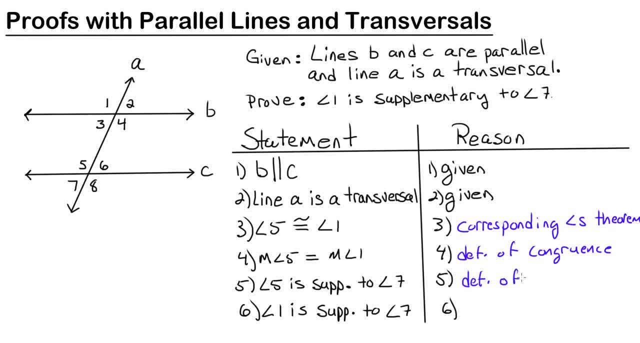 Statement 5 says angle 5 is supplementary to angle 7, let's take a look at them: here's 5, here's 7, and together they make a straight line. so we know they're supplementary because they are a linear pair, and that's our reason is definition of linear pair. 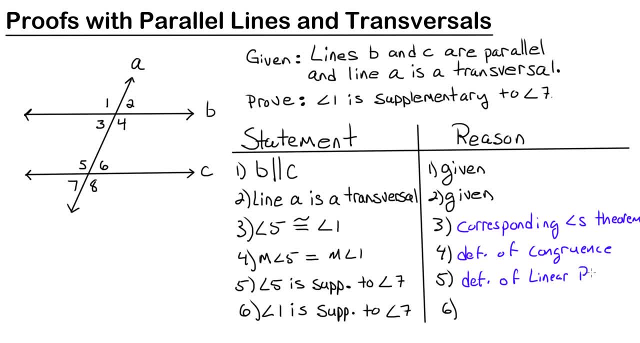 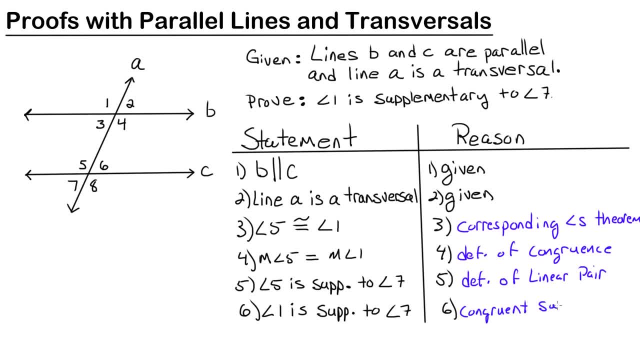 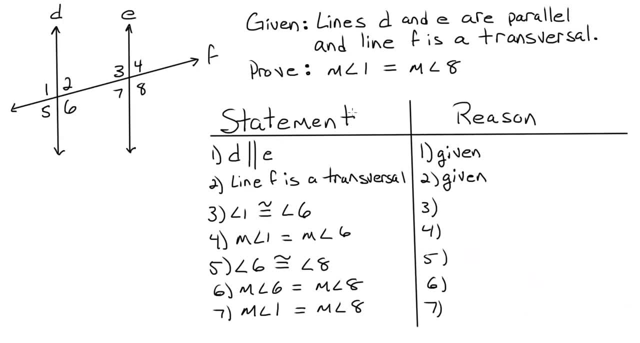 Statement supplements theorem. So our next example says: given lines D and E- here they are- are parallel and line f is a transversals, prove that the measure of angle 1 is equal to the measure of angle 8.. So let's look at our statements and reasons. 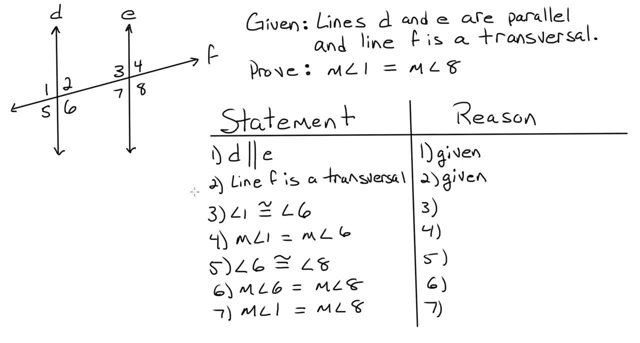 Number 1, D is parallel to E. that's given Number two. line F is a transversal. that is also given. Statement three: angle one is congruent to angle six. If we look at them we can see that they are vertical. 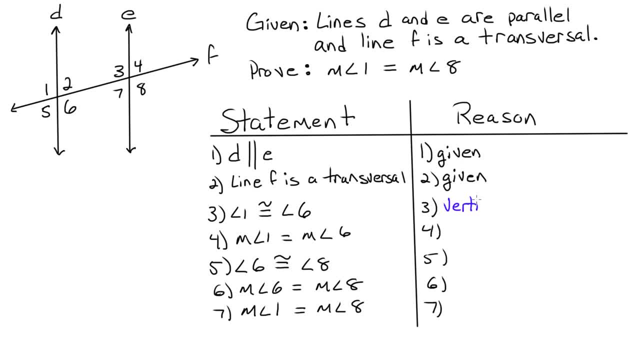 So we know they're congruent because of the vertical angles theorem. And since they are congruent, we know that the measure of angle one is equal to the measure of angle six. So that is the definition of congruence. Statement five says angle six is congruent to angle eight. 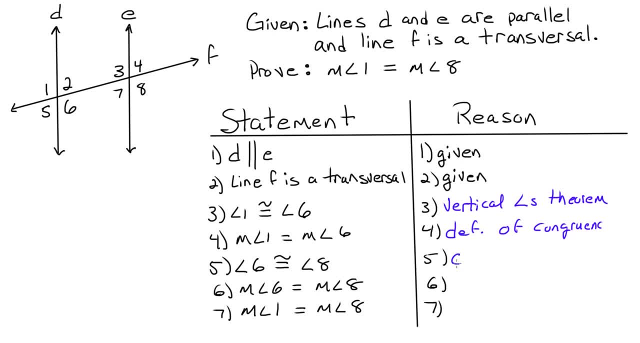 And we see that that is because they are corresponding. So that is the corresponding angles theorem. That tells us that the angle six is congruent to the angle eight. That tells us that the measure of angle six is equal to the measure of angle eight. 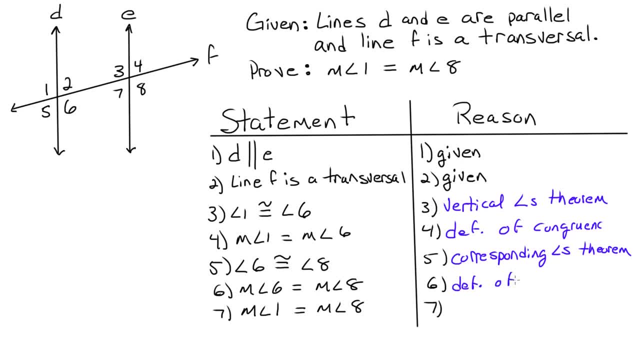 Again, the definition of congruence. Now there's a property in mathematics that tells us that if A equals B and B equals C, then A also equals C, And that is called the transitive property. And that is what's happening here. 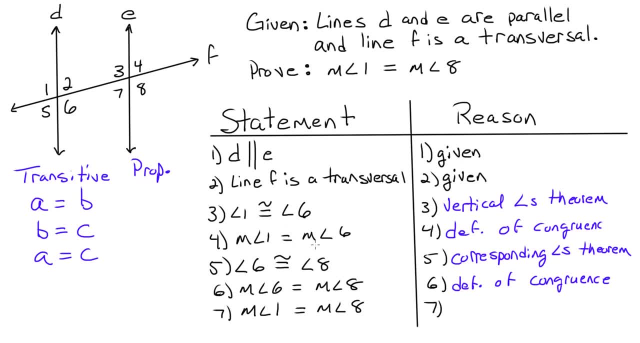 You see, we've shown that the measure of angle one is equal to the measure of angle six. Then we showed that the measure of angle six is equal to the measure of angle eight. So if one equals six and six equals eight, that means the measure.